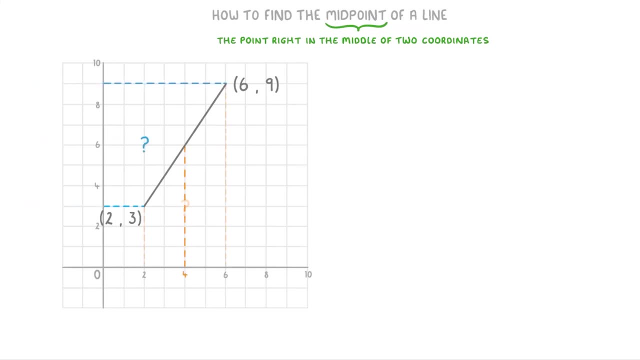 of the midpoint. we just need to find what's in the middle of 3 and 9,, which is 6.. So the midpoint is 4, 6.. Now this one here was a fairly easy example, and we had the graph. 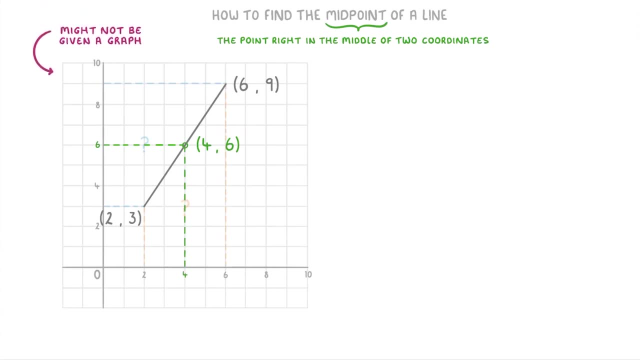 to help us In exams, though you might not have the graph and the numbers involved might be a bit more complicated, So a better technique to find the midpoint is to use this formula instead. It works in basically the same way by finding the average of the x-values and. 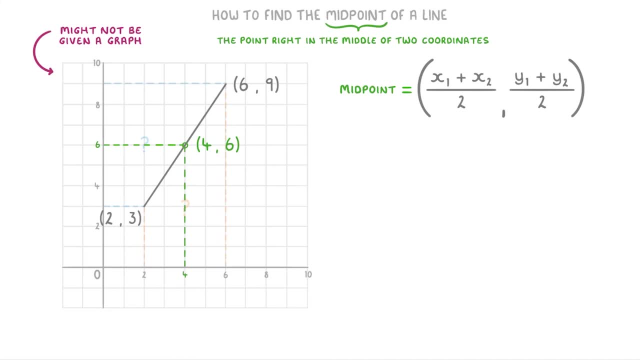 the average of the y-values. But before we can use it we need to label our two points. So we pick one of them to be the first and label the coordinate, and the other point to be the second and label the coordinate, although it doesn't. 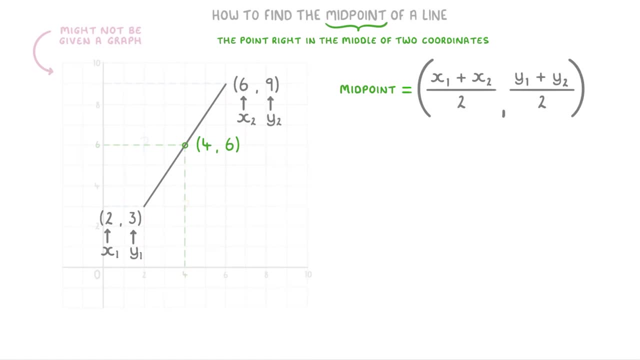 matter which point is the first and which point is the second. Then, to use our formula, all we have to do is plug in the numbers. So we start by adding together x1 and x2, and then we divide it by 2 to get the average of those two x-coordinates, which will be 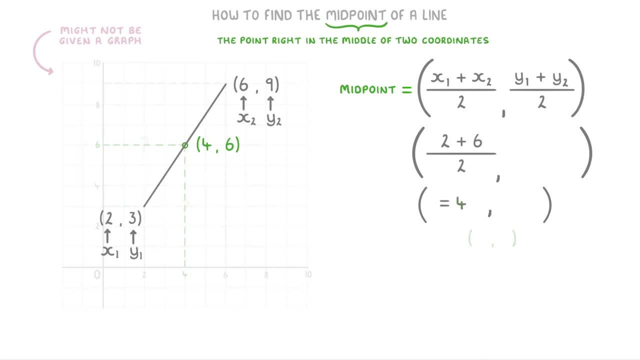 4.. And so we know that the x-coordinate of our midpoint is 4.. Then we do exactly the same thing with the two y-values, So we do 3 plus 9, divided by 2,, which is 6.. So that's. 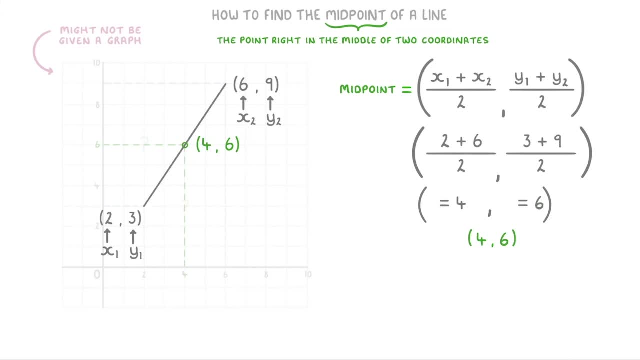 the y-coordinates of our midpoint And notice that we've got a final answer of 4, 6,, just like we did when we used our formula. Now, if we take a closer look at this formula for a moment, you might notice that it's actually. 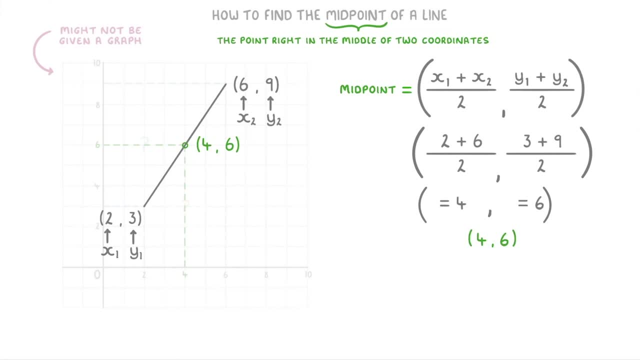 written like a pair of coordinates, which is why it has the brackets on the sides and the comma in the middle. So this left part is basically a mini-formula to work out the x-coordinates of the midpoint by finding the average of our x-values and this right part. 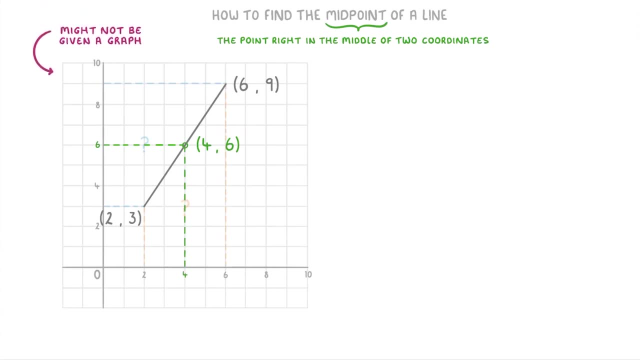 to help us In exams, though you might not have the graph and the numbers involved might be a bit more complicated, So a better technique to find the midpoint is to use this formula instead. It works in basically the same way by finding the average of the x values and. 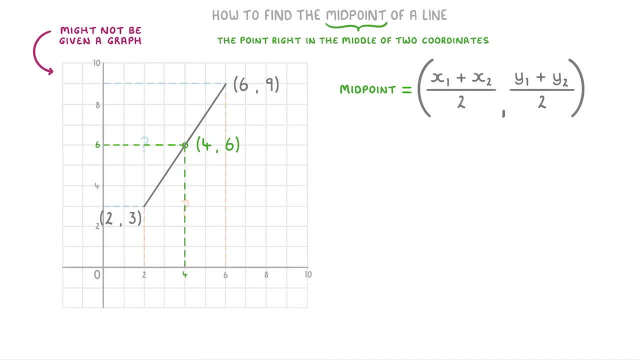 the average of the y values. But before we can use it we need to label our two points. So we pick one of them to be the first and label the coordinate x1, y1, and the other point to be the second and label the coordinate x2, y2.. Although 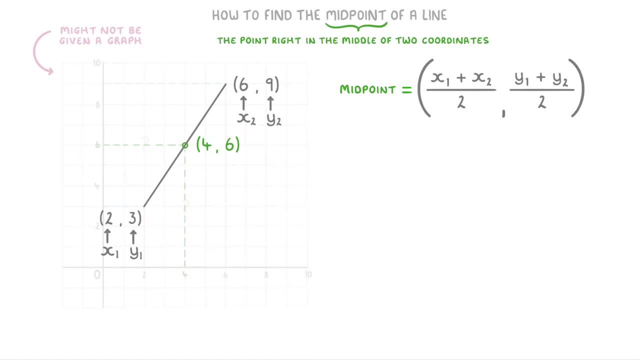 it doesn't matter which point is the first and which point is the second. Then to use our formula, all we have to do is plug in the numbers. So we start by adding together x1 and x2,, which would be 2 plus 6.. 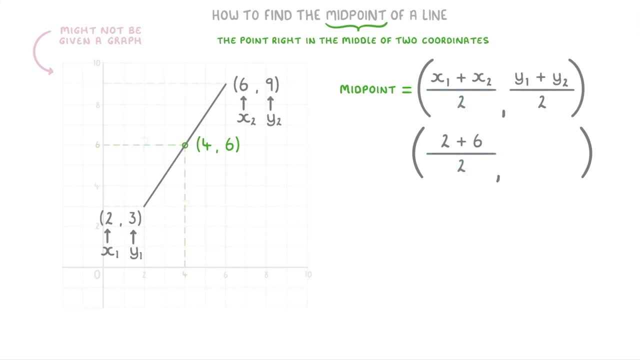 And then we divide it by 2 to get the average of those two x coordinates, which will be 4.. And so we know that the x coordinate of our midpoint is 4.. Then we do exactly the same thing with the two y values. So we do 3 plus 9, divided by 2, which is 6.. So that's. 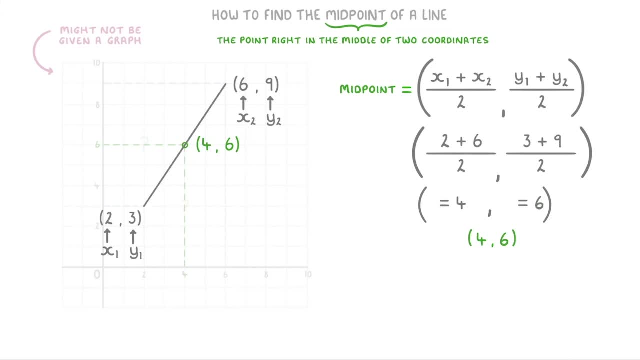 the y coordinates of our midpoint And notice that we've got a final answer of 4, 6,, just like we did when we used the formula for the first and the second. Now, if we take a closer look at this formula for a moment, you might notice that it's actually 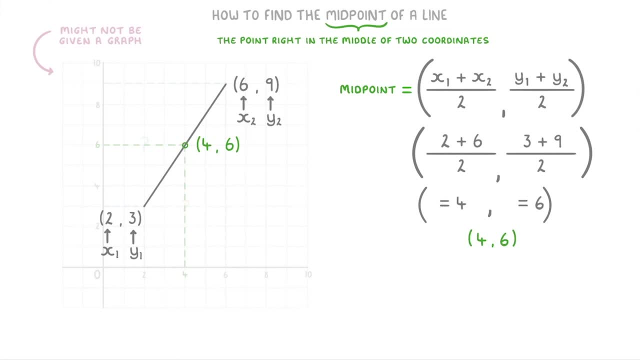 written like a pair of coordinates, which is why it has the brackets on the sides and the comma in the middle. So this left part is basically a mini-formula to work out the x coordinate of the midpoint by finding the average of our x values. And this right part is a mini-formula to work. 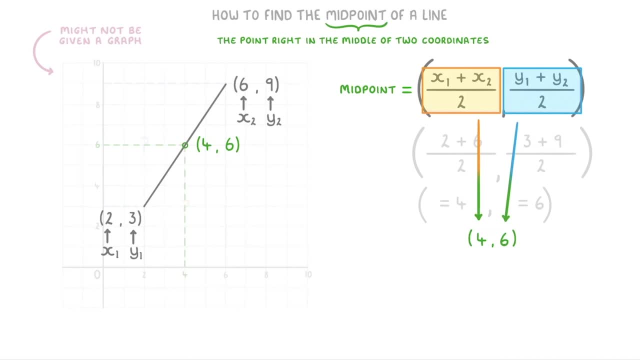 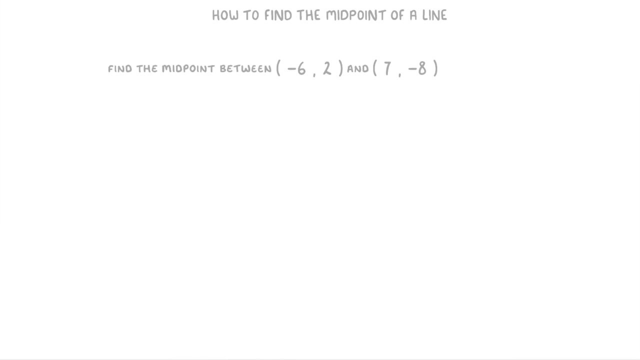 out the y coordinates By finding the average of our y values. So this is why we just plug everything straight in, and when we simplify it, we end up with the coordinate that we need. Let's try one more question, from scratch this time. So here we're looking for the midpoint.